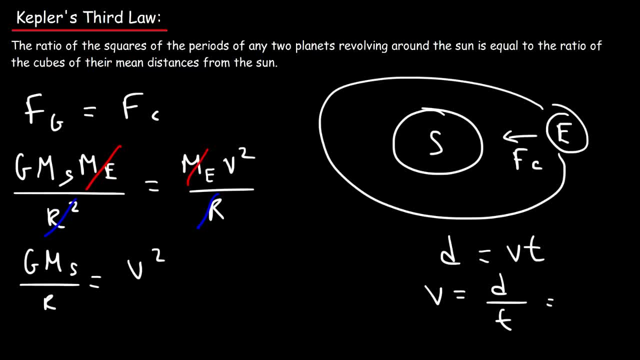 earth is traveling in a nearly circular orbit, so the distance around a circle is 2 pi R. the time it takes to revolve around that circle is the period. so therefore we can replace V squared with 2 pi R over T squared- it's not me- and make some more space. so we now have is G times the mass of the. 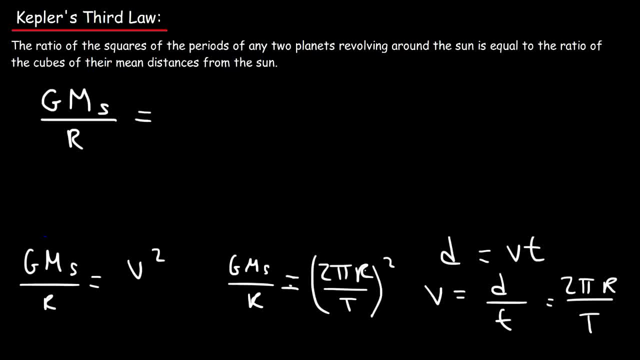 Sun over R is equal to if we square both sides- or not both sides, but just this side- 2 squared is 4, and then we're gonna have pi squared times, R squared over T squared. now let's cross multiply. so on the left we're gonna have G times, MS times T. 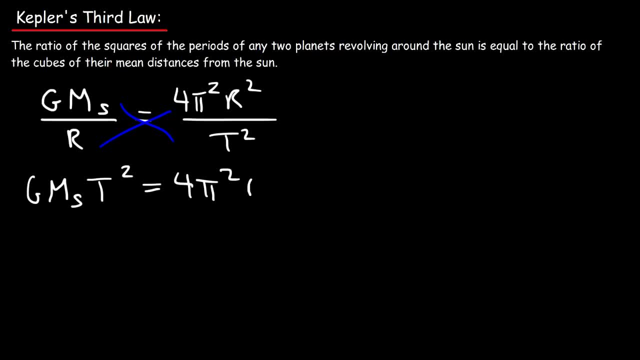 squared is equal to 4 pi squared times R cubed. now save this portion of the equation in this form. we're going to use it later in this video, so just make a note of it. now i'm going to solve for T squared, so I need to divide both sides. 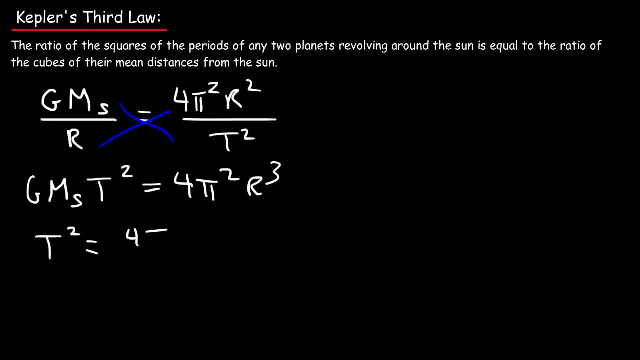 by GM. so T squared is 4 pi squared over R squared. squared, R cubed over G times M. Now what I'm going to do is divide T2 squared by T1 squared, So T2 is going to be 4 pi squared, R2 raised to the third over GMS. 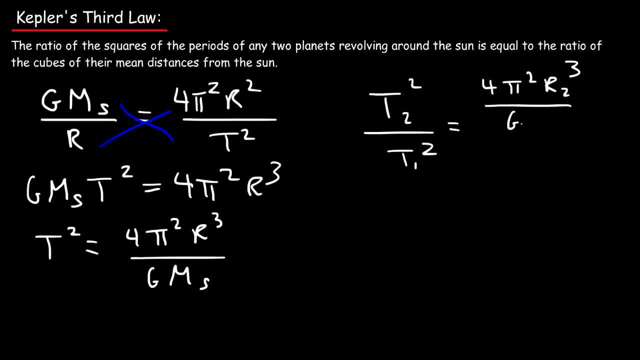 based on this equation, T1 squared is going to be 4 pi squared, R1 cubed over GMS, So G and the mass of the sun is going to be the same, so we can cancel it, And 4 pi squared is going to be the same, So we're left with T2 squared over T1 squared. 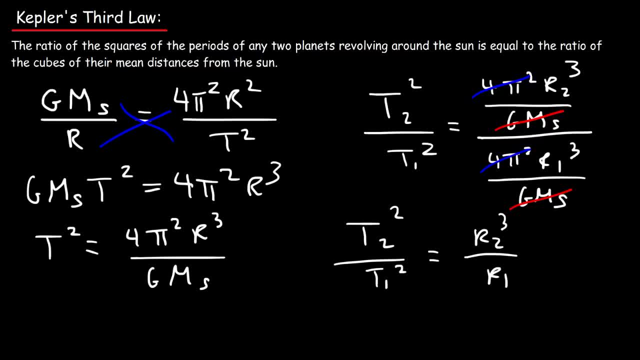 and that's equal to R2 squared, R2 cubed over R1 cubed, which, if we want to, we can write it as T2 over T1 raised to the second power, equals R2 over R1 raised to the third power. 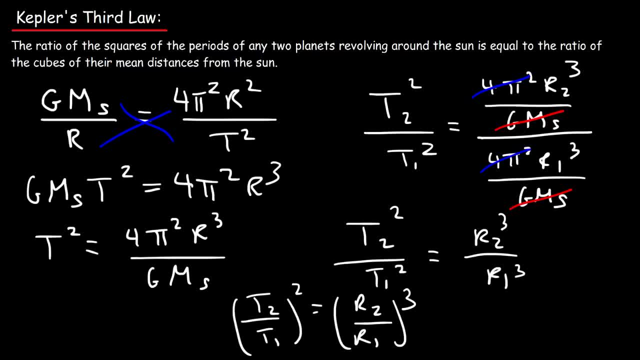 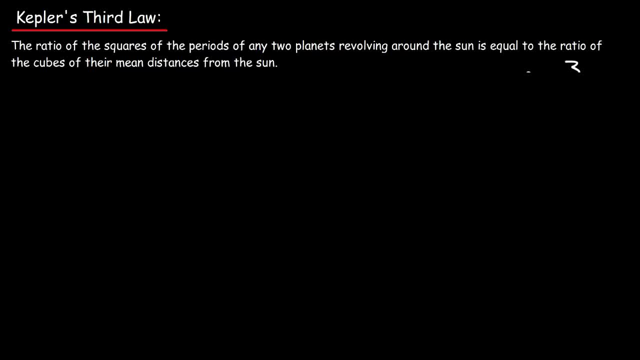 So that's how you can derive the equation that's associated with Kepler's third law. Now let's work on a few practice problems. The mean distance: The mean distance between the earth and the sun is 1.5 times 10 to the 11 meters. 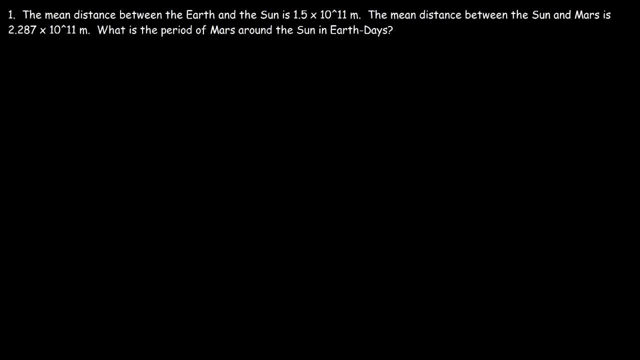 The mean distance between the sun and Mars is 2.287 times 10 to the 11 meters. What is the period of Mars around the sun in Earth days? So let's say: this is the sun, Here's the earth And here's Mars. 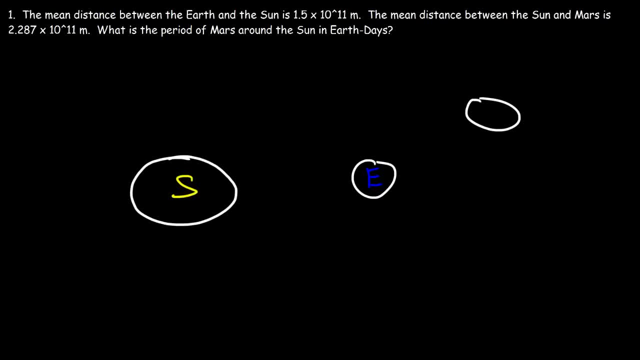 So let's say this is the orbit for Earth and this is the orbit for Mars. Now it takes Earth 365 days to orbit the sun And it takes Mars some unknown number of days to orbit it. So let's say this is the orbit for Mars. 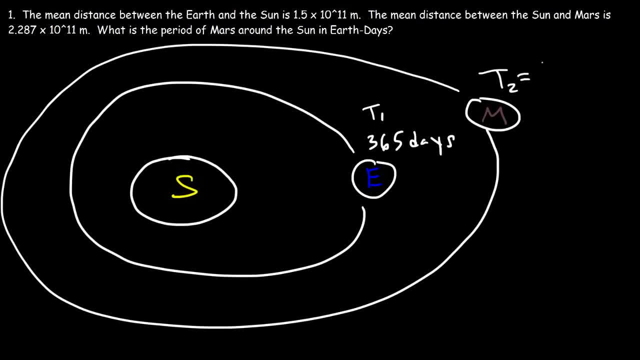 So let's say if this is T1, we need to find T2.. That's the time it takes for Mars to orbit the sun. Now we have the mean distance between the center of the earth and the center of the sun. That's about 1.5 times 10 to the 11 meters. 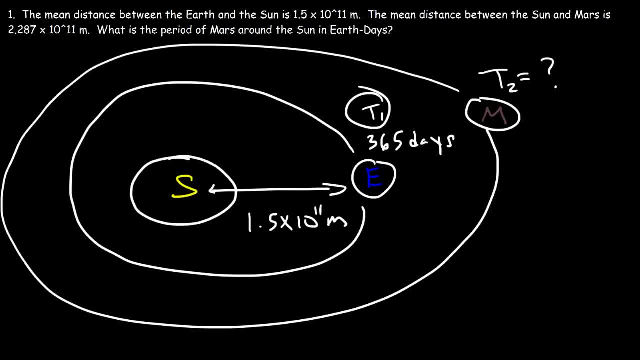 So if T1 corresponds to earth, R1 has to be the distance between the sun and the earth. Now the distance between the sun and the earth is 1.5 times 10 to the 11 meters The sun and Mars that's given to us. 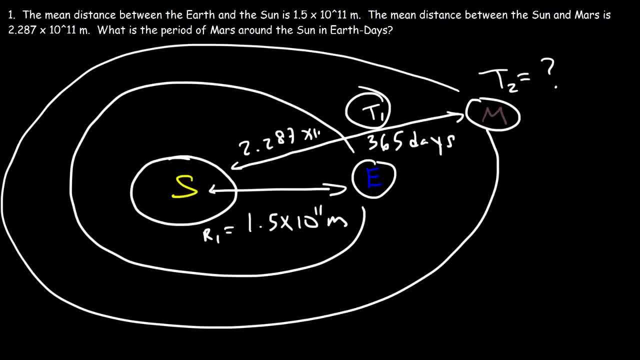 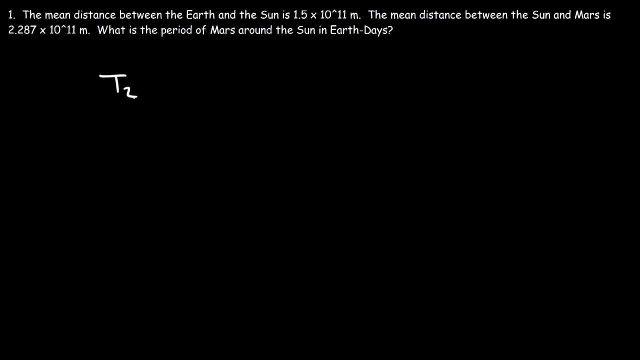 That's 2.287 times 10 to the 11.. So we're going to define that as R2.. Our goal is to calculate T2.. So T2 over T1 squared is equal to R2 over R1 cubed. 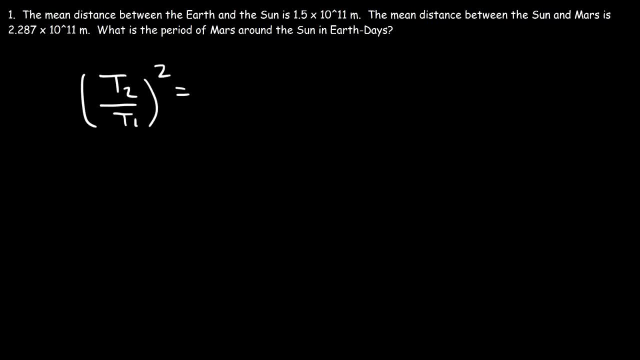 Or, if you want to, you can write it down. You can write it this way. It might be easier to do it like this: T2 squared over T1 squared is equal to R1 cubed, with R2 cubed on top. 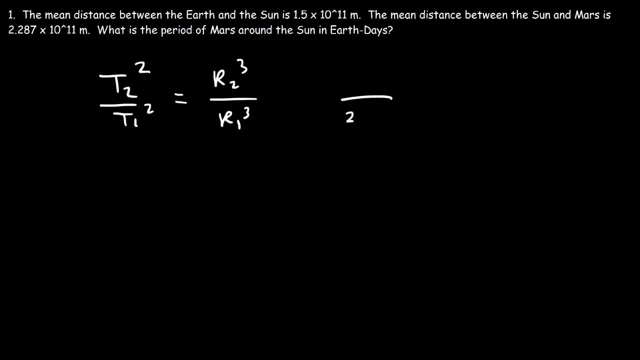 So let's say that T1 corresponds to the earth. So it's 365 days squared And we're looking for T2. So R1 is 1.5 times 10 to the 11.. And let's raise that to the third power. 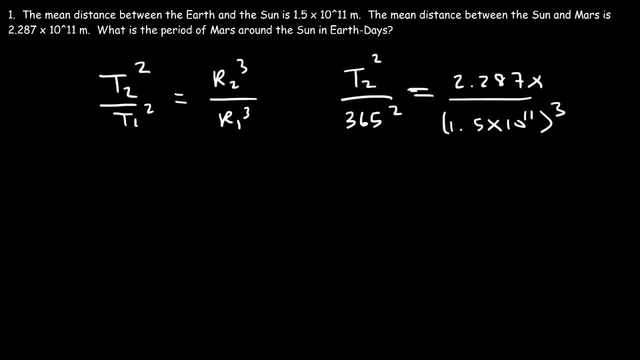 R2 is 2.287 times 10 to the 11 to the third power. So let's cross multiply first. So on the left I'm going to have 365 squared times 2.287 times 10 to the 11, raised to the third power. 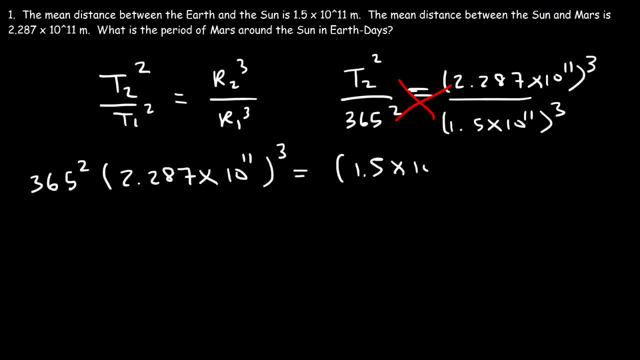 And on the right it's going to be 1.5.. Times 10 to the 11, raised to the third power Times T2 squared. Now I'm going to divide both sides by this number, So I'm no longer going to have it on the right side. 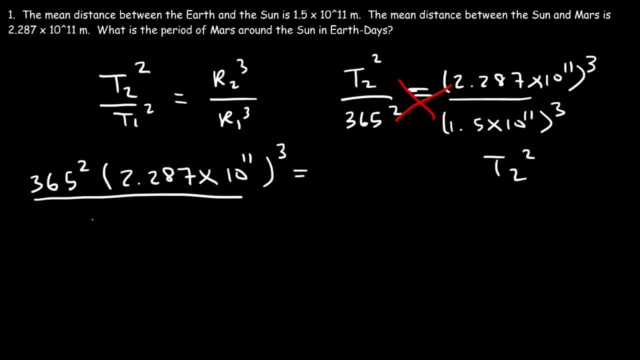 But it's going to be on the bottom of the left side. So now let's type this in: And to calculate T2 squared, So 472,183.1.. That's equal to T2 squared. So now we need to take the square root of both sides. 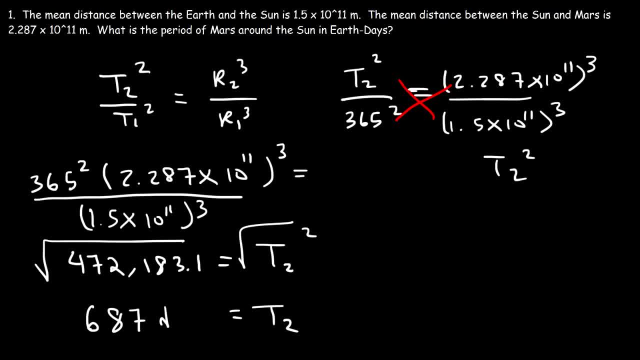 So T2 is about 682.. 682,187 days, So that's how long it takes Mars to orbit the sun. So one year on Mars is 687 days. That's a long time. One year on the Earth is 365 days. 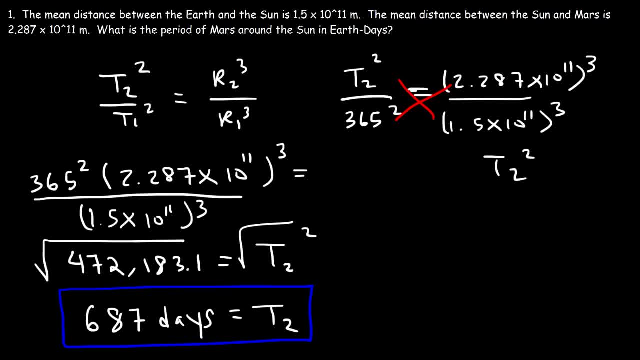 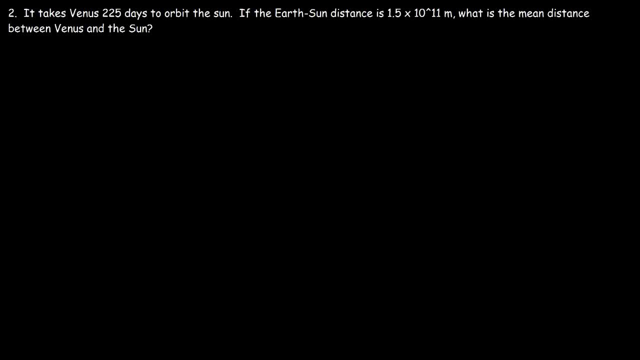 A year is defined as the time it takes for a planet to orbit the sun. Now let's move on to the next problem. It takes Venus 225 days to orbit. So if you're going to take it to the sun, If the Earth-Sun distance is 1.5 times 10 to 11 meters- 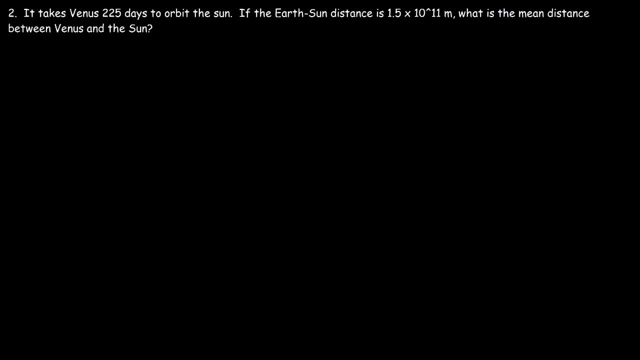 What is the mean distance between Venus and the sun? So if you want to draw a picture, Let's say this is the sun And here is the Earth, And let's say here's Venus. So this is the orbit for Venus And this is the orbit for the Earth. 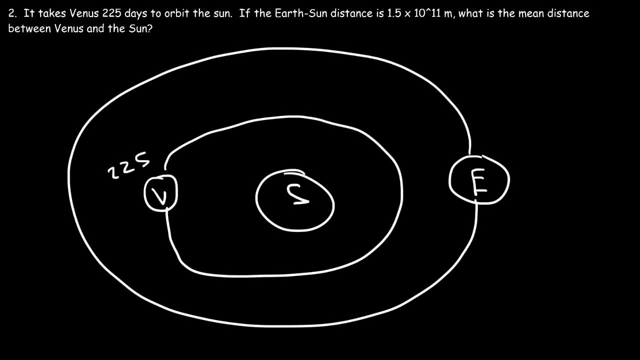 So it takes Venus- it's 225 days because it's closer to the Sun, for the earth is 365 days. we know the distance between the Sun and the earth: it's 1.5 times 10 to 11. we need to find the distance between Venus and the Sun, so let's call it r2. that's the 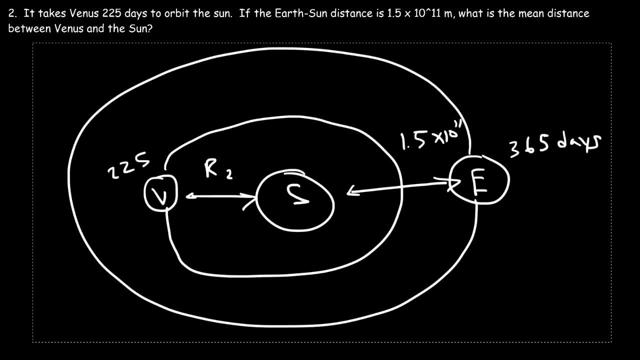 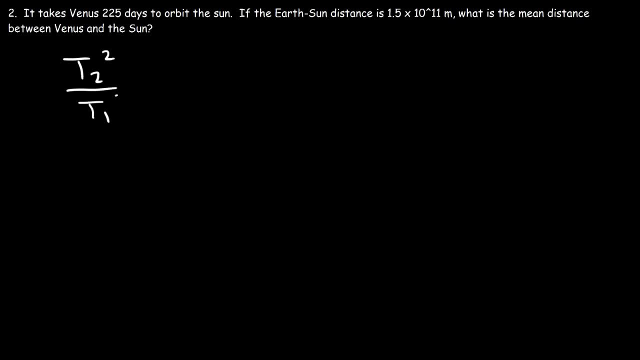 missing variable that we're looking for. so, using the same equation, t2 over t1 squared is equal to r2 over r1 cube. so t1- we're going to apply it for earth, that's going to be 365 days, and t2- that's going to correspond for the 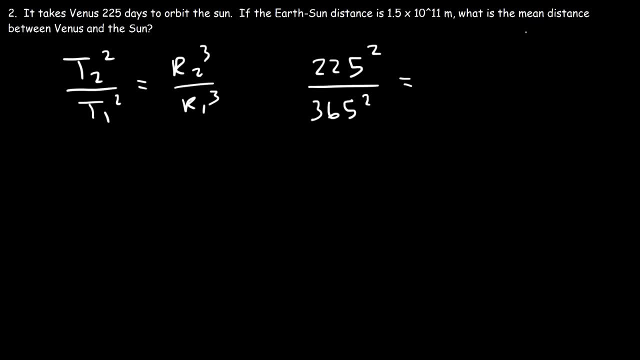 period for Venus, which is 225 earth days. r1 is 1.5 times 10 to 11, raised to the third power. so we're looking for r2 in this problem. so, just like before, we're going to cross, multiply, so it's going to. 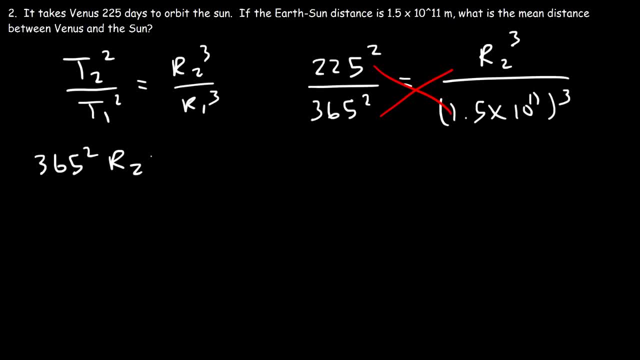 be 365 squared times r2 cube, and that's equal to 225 squared times 1.5 times 10 to 11 raised to the third power. so I'm going to divide both sides by 365 squared. so r2 raised to the third power it's going to be 1.5 times 10 to 11 raised to. 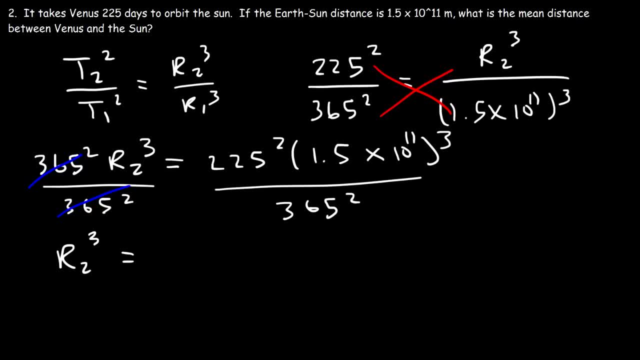 the third power times 225 squared divided by 365 squared. so you should get 1.28 to times 10 to the 33. now to get our raised both sides to the 1- 3rd power. so r2 is the cube root of that number, which 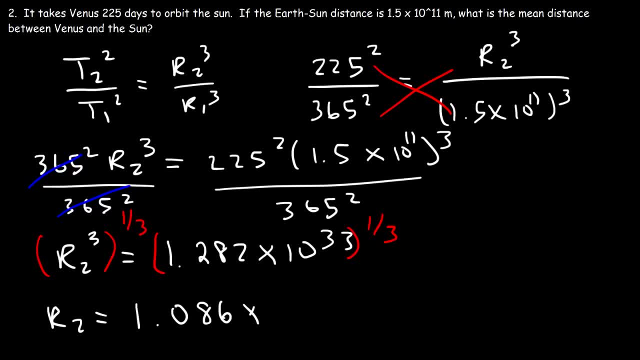 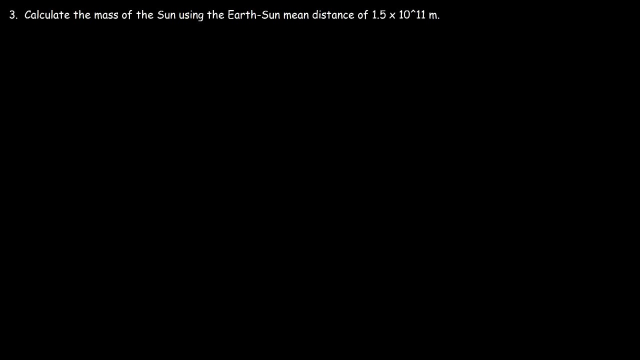 is 1.086 times 10 to the 11 meters. so, as you can see, it's less than the Earth Sun distance, because Venus is closer to the Sun and so it's going to have a smaller period. number three: calculate the mass of the Sun using the Earth Sun mean. 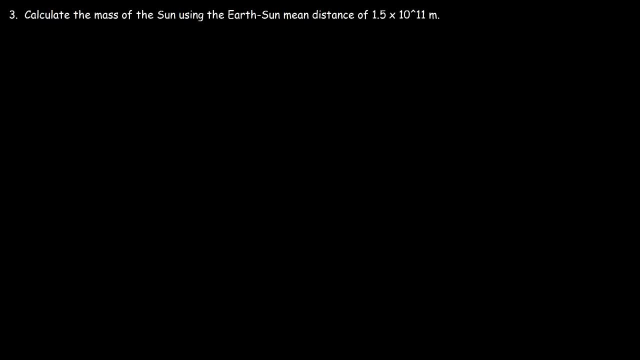 distance of 1.5 times 10 to 11. now, earlier in this video I mentioned to highlight this equation which we derived already: G times MS T square is equal to four pi squared r cube. so we divide this equation where the Sun was at the 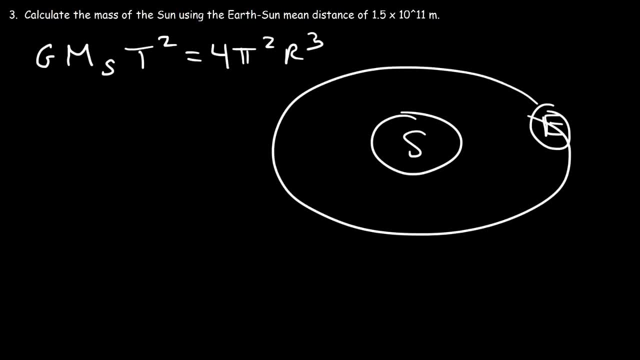 center and the earth was orbiting the Sun. we sent this a triple force equal to the gravitational force, and we also replace the velocity with 2 pi r over T, and we were able to get this equation. now, all we got to do from that point is: 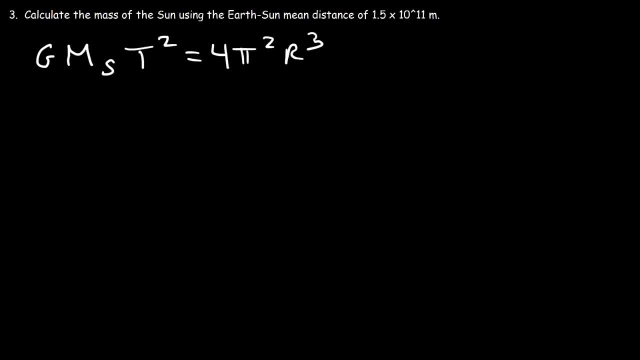 solve for M, that's going to give us the mass of the Sun. so to do that we need to divide both sides by G T squared, so the mass of the Sun can be calculated using this equation. it's four pi squared times r, raised to the third power, divided by G T squared. so if you need to find the 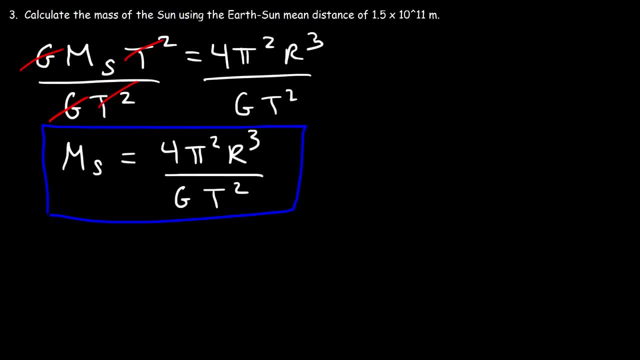 mass of any planet or the mass of the Sun. you can use this formula where T is the time it takes for an object to orbit the Sun or that planet. so let's say, if you want to find the mass of the Earth, you want to use the period of the moon, because you need. 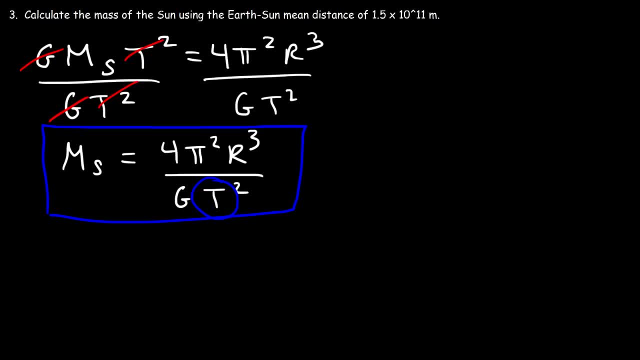 a satellite that's orbiting it. if you want to find the mass of the Sun, the earth is acting like a satellite because the earth is orbit in the Sun, so you would have to use the period of the earth if you want to find the mass of the. 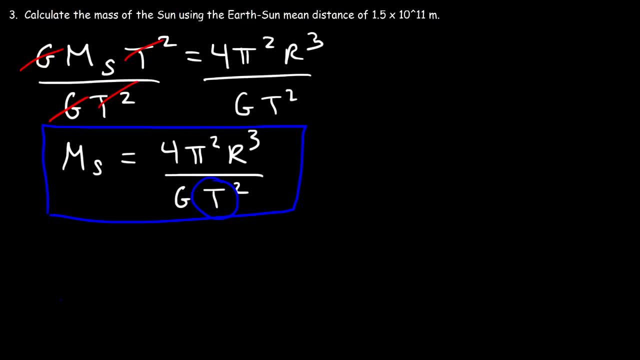 earth. use the period of the moon for T, so let's go ahead and plug everything we have. so r is the distance between the earth and the Sun. that's 1.5 times 10 to 11th, raised to the third power, and G is: 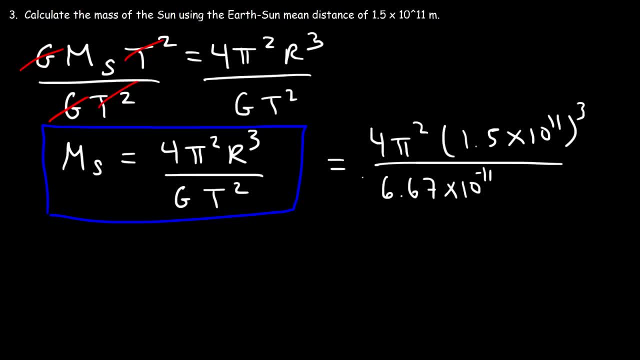 six point six, seven times 10 to the minus eleven, and T is the period of the earth and T is the period in seconds. now it takes about 1 year for the earth to travel around the Sun, so that's about 365 days now if you want to incorporate. 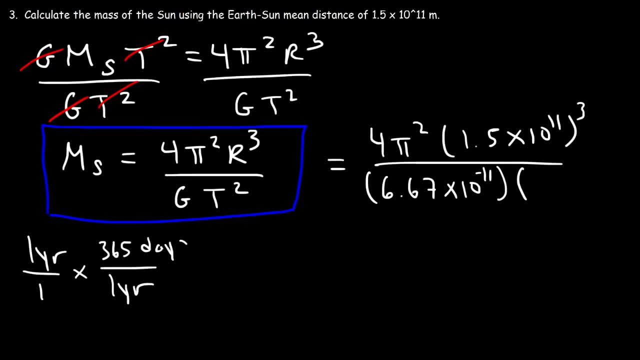 the leap year and say 365, point two: five days. that's fine too, but the answer is not going to change much, it's going to be about the same. each day contains 24 hours, and each hour is 60 minutes, and one minute is equivalent to 60 seconds. so we 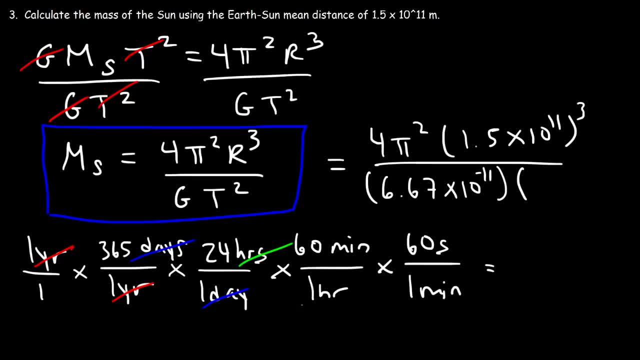 can cancel the unit days, hours and minutes. so it's 365 x 24 x 60 x 60, so it takes the earth 31 million five hundred and thirty six thousand seconds to orbit the Sun. and don't forget to square that number, so you should get. 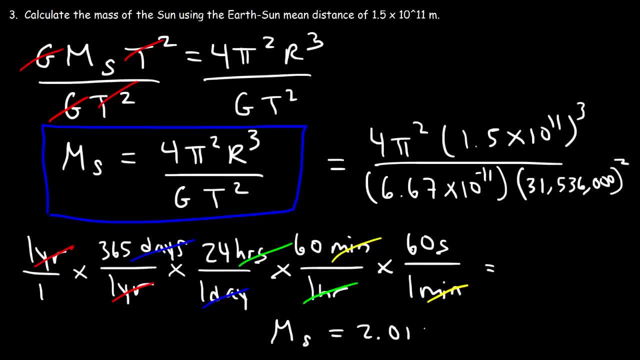 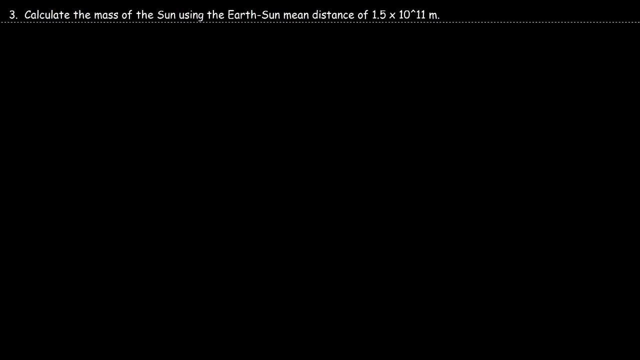 2.01 x 10 to the 30 kilograms. so that's the mass of the Sun. so let's say, if you want to calculate the mass of the earth using that same formula, now, in order to calculate the mass of the earth, the earth has to be the object. 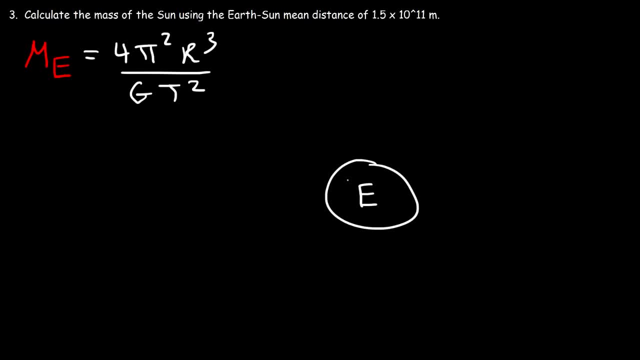 in the center. so we need something that's orbit in the earth. in this case, we're going to use the moon. so we need two things: the Earth- moon distance, which you can look it up. so we need two things: the Earth-Moon distance, which you can look it up, that's about relax, but sun and moon distance on the. 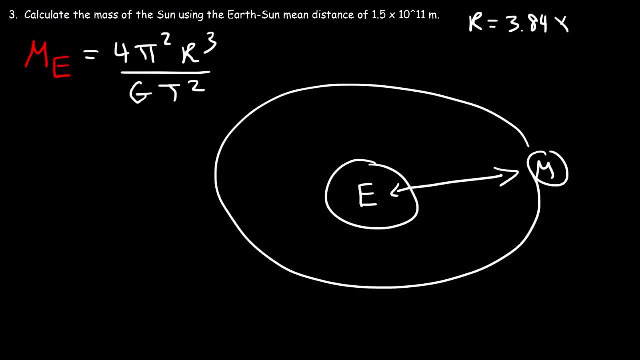 It's about 3.84 times 10 to the 8 meters and you need the period of the Moon. It takes the Moon about 27.4 days to orbit the Earth. Now we need to convert that value to seconds. So t is 27.4 days and 1 day is equivalent to 24 hours. 1 hour is 60 minutes and each 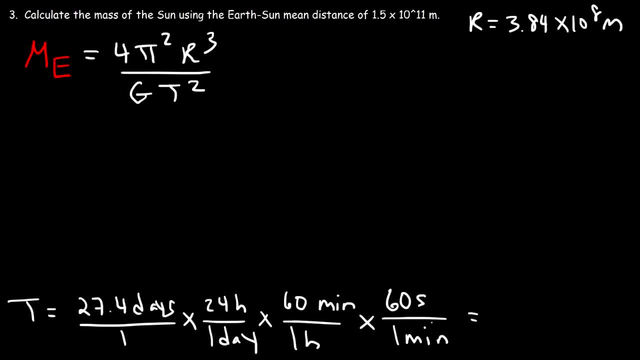 minute is equivalent to 60 seconds, So it's 27.4 times 24 times 60 times 60.. So the period is 2,000,000.. 367,000, and 360 seconds, So that's how long it takes the Moon to orbit the Earth. 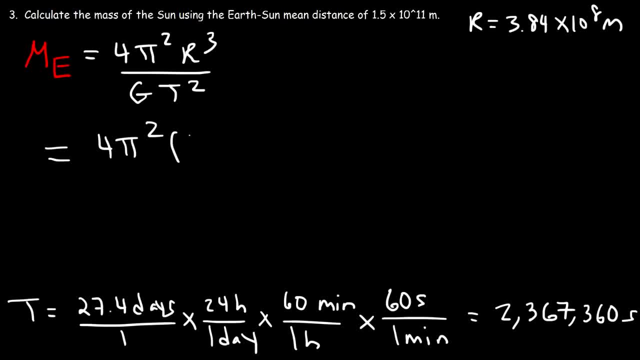 So now we can plug in everything. So it's 4 pi squared times 3.84 times 10, to the 8 meters raised, to the third power divided by the gravitational constant multiplied by 2,367,360 squared. So go ahead and do that. 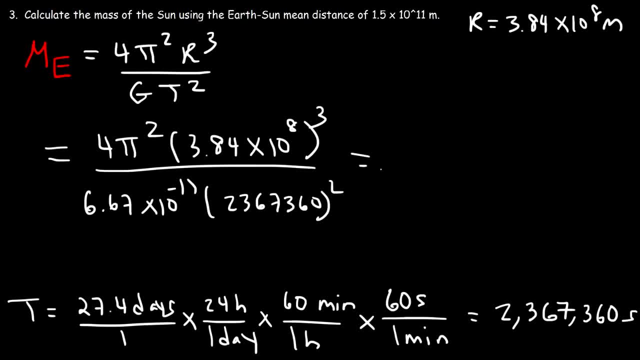 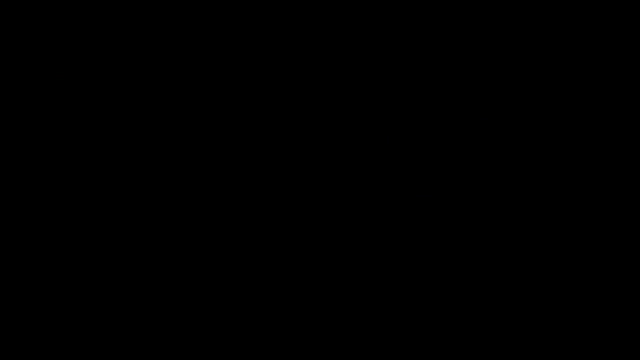 Go ahead and type this in, So you should get about 5.98 times 10 to the 24 kilograms, which is the mass of the Earth, And then you can do a little bit more. It takes the total to the third power. 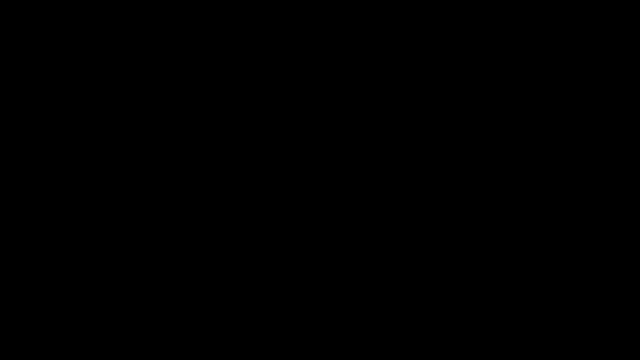 So let's do that. So it's 1,000,000.. It's a little bit more than 4 pi squared plus 1,000,000.. So the time that the Moon will move is approximately 1,000,000.. So the time is about 1,000,000 for the Earth and 1,000,000,000 for the base.